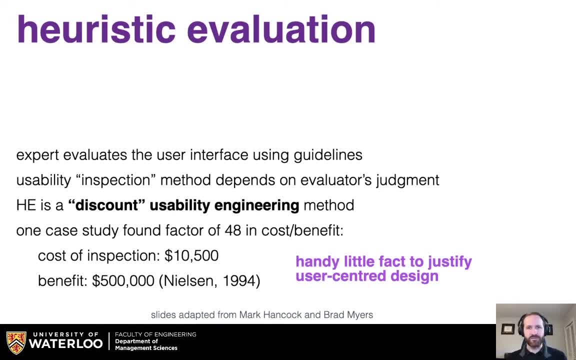 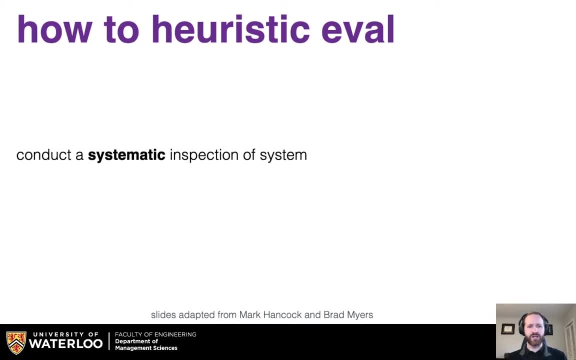 and think about using these design methods and creating effective interfaces and systems. So how do you conduct a heuristic evaluation? Well, you conduct a systematic inspection of a system. You want multiple evaluators- that's way better, And you want trained evaluators if possible. 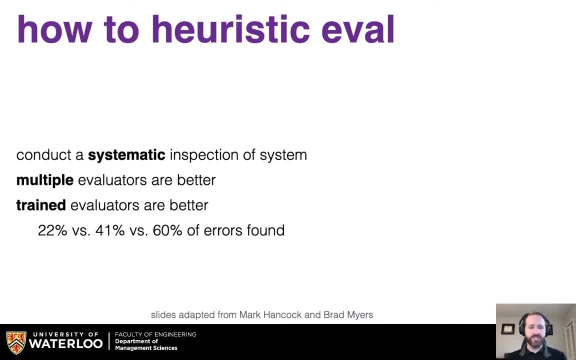 that's way better, And what you get is increasingly more errors found: 22% for a single systematic inspection of a system, 41% for multiple evaluators and 60% for trained evaluators. They go through the entire interface, the whole interface. 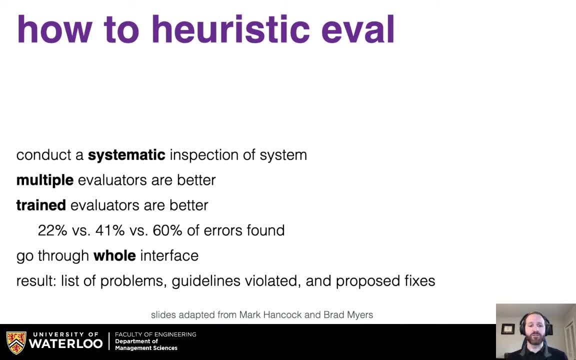 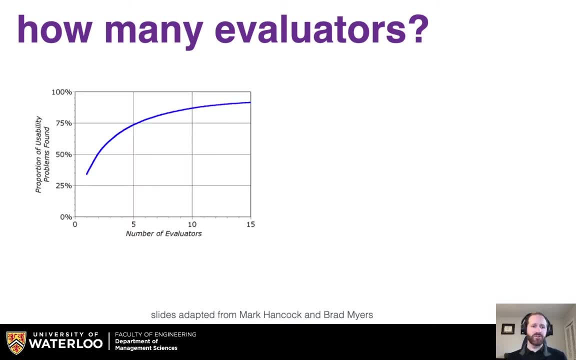 and the result is a list of problems, guidelines violated and proposed fixes. So how many evaluators should you recruit? Well, work by Nielsen shows that as you increase the number of evaluators, you catch more errors, but it starts to plateau. 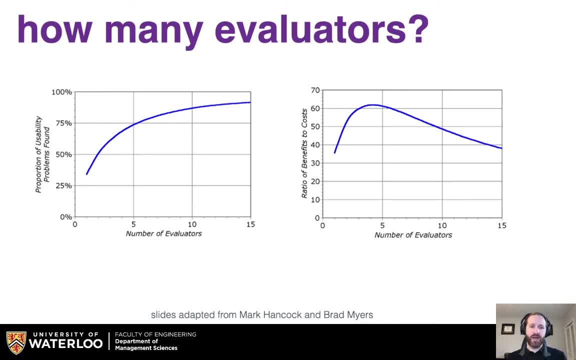 reaches a bit of an asymptote And you have a a reduction in the benefits to cost, because as you increase the experts, your costs increase, but your benefits are starting to decrease. And so Nielsen suggests that four might be optional And that gets you, you know, about 70% of errors. 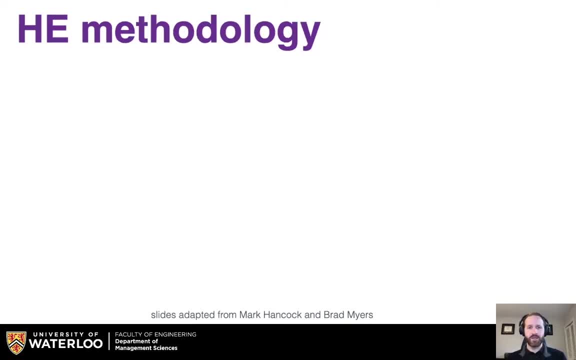 but also keeps the cost benefit pretty high. So we're gonna go through the heuristic evaluation methodology. The reference is Nielsen's How to Conduct a Heuristic Evaluation at this link. Take a look at this, especially as you go through your heuristic evaluation assignment. 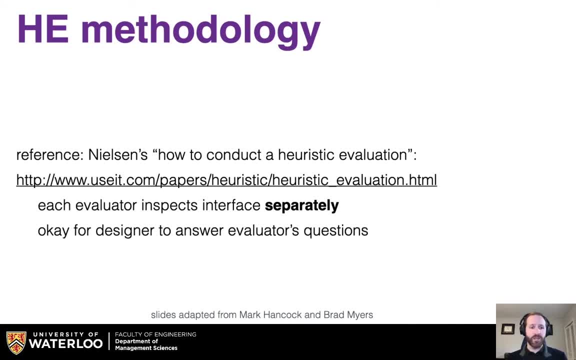 Each evaluator inspects the interface separately and it's okay for the designer to answer the evaluator's questions. They're an expert, They're gonna weigh all these things in their opinion And you go through the interface several times using the heuristics. 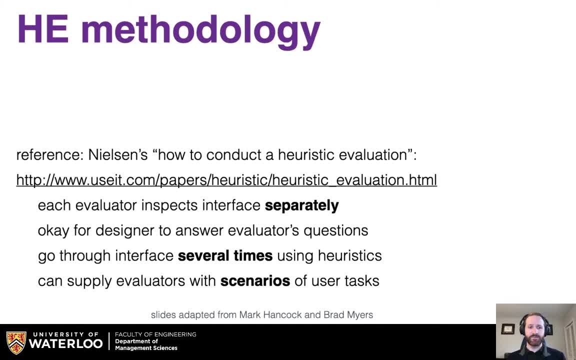 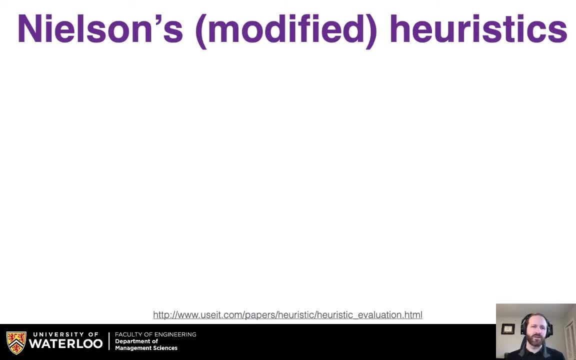 You can also supply evaluators with scenarios of user tasks, And what you do is you provide a set of heuristics. We'll go through Nielsen's modified heuristics. These ones have been evaluated and refined over the years. The first one is visibility of system status. 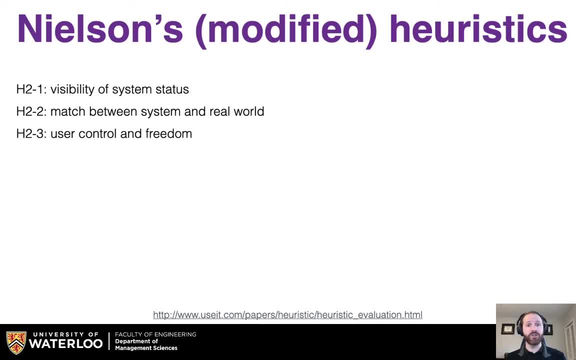 You've got match between the system and the real world, user control and freedom, consistency and standards. error prevention, recognition rather than recall, flexibility and efficiency of use. aesthetic and minimalist design help users recognize, diagnose and recover from errors. 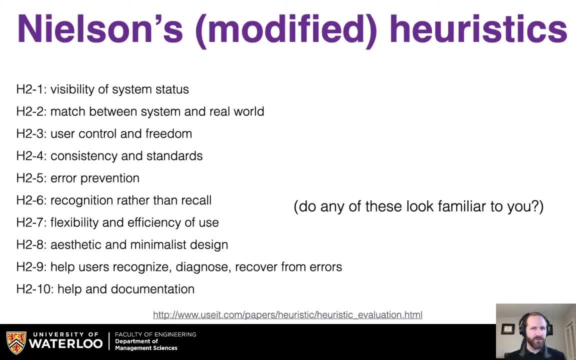 and help and documentation. Do any of these look familiar to you? Many of these are tied to the interaction design principles that we've discussed in the class and from some of the outcomes from our discussion of cognitive properties and of human capabilities. So they're all grounded in the literature. 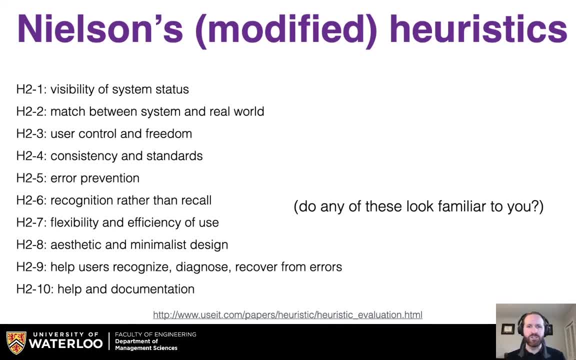 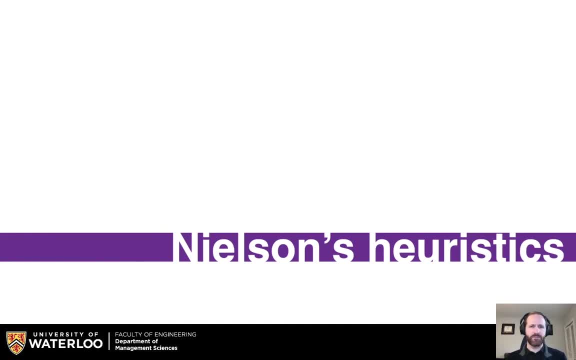 and the work that we've already looked at and this kind of ties them together in a systematic way to do an effective evaluation of a system. Let's go through each of Nielsen's heuristics in a little more depth. The first one is visibility of system status. 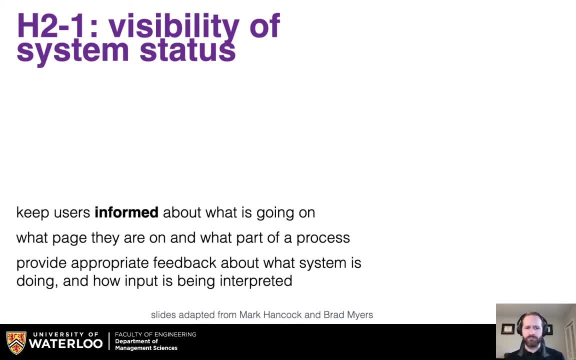 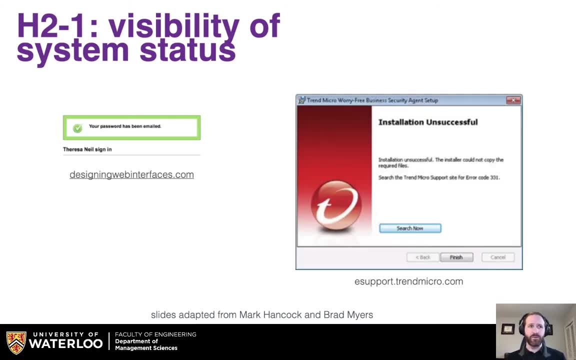 You wanna keep users informed about what is going on, what page they're on what part of the process. You wanna provide appropriate feedback about what the system is doing and how input is being interpreted. So, for example, you wanna have a confirmation at the end. 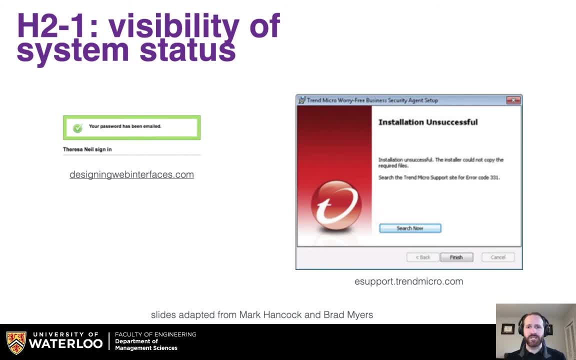 saying yes, your password has been emailed. once you've signed in or you've forgotten your password, or if something was unsuccessful, you have that visibility that the system did not install whatever you wanted to install. The second heuristic is match between the system. 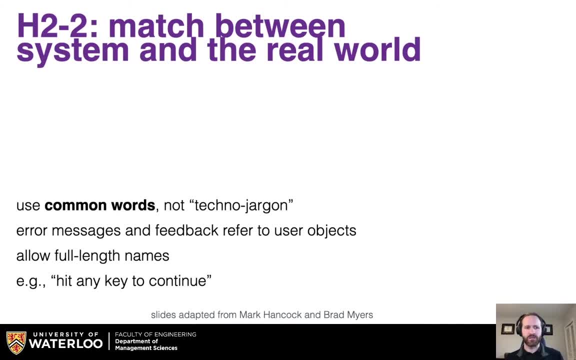 and the real world. You wanna use common words and not techno jargon. You wanna have error messages and feedback that refer to user objects- things that the user and other people involved in the system will understand. You wanna allow for full length names. 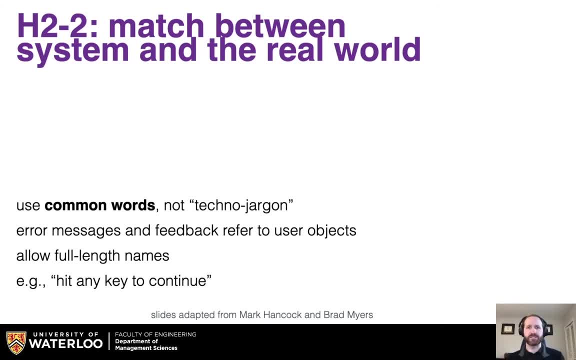 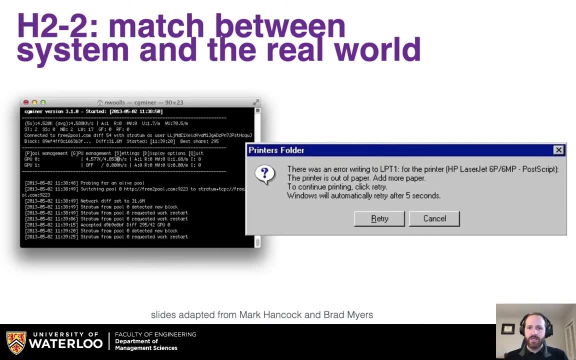 So if you're gonna see things like hit any key to continue, you want that full text to allow people to understand what it means. You know? oh, any key. Okay, I press any key. So some examples might be you know. 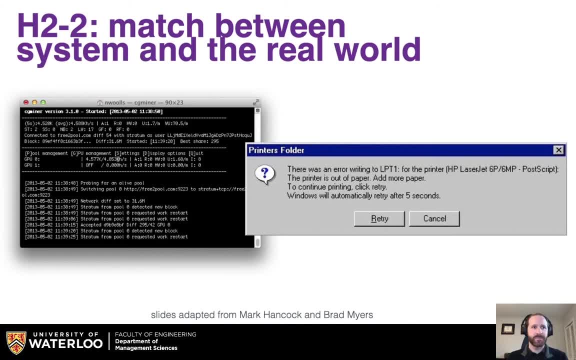 this one on the left where you've got a terminal interface and you have a bunch of this really jargony, difficult to understand- feedback. This might be useful if you're, you know, an expert expert diagnosing the system. usually you can access a screen like this, but the one 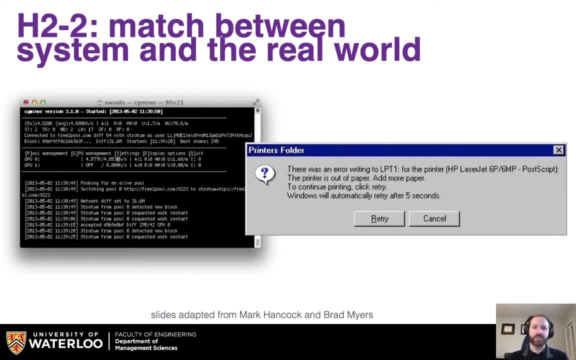 on the right has a lot more match with the real world. It says that there's an error running to the printer. it gives an example, a full name of the printer. it says it's out of paper and you need to add more paper and then to 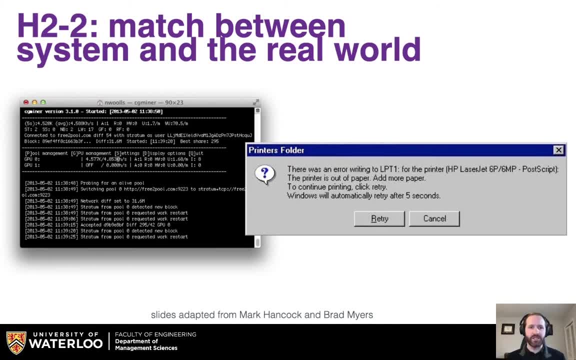 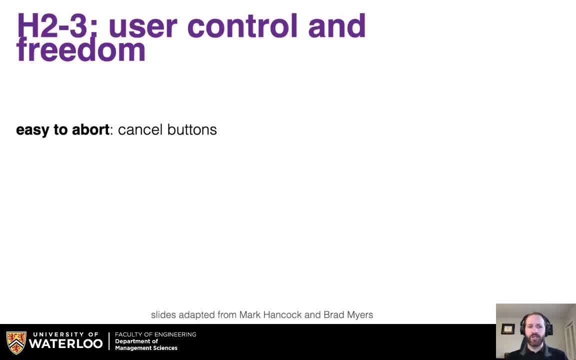 continue printing, click retry. so it's got all of this extra information explained quite clearly and related to the real world. The third heuristic is user control and freedom. You want things to be easy to abort. you want to have cancel buttons, things like that. 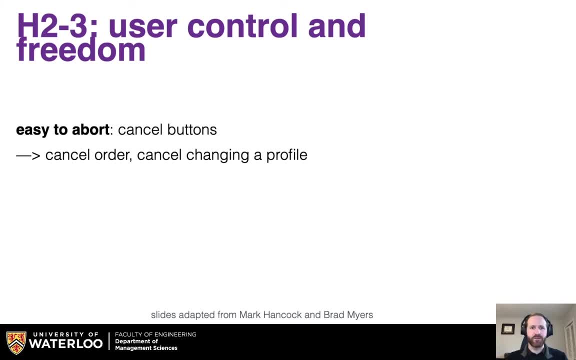 You want to be able to cancel an order, cancel changing a profile. if you're in a screen that you don't want to be in, you want to be able to get out of that. You want to have things be easy to undo. 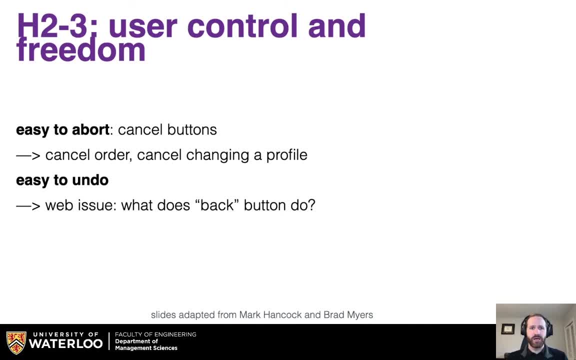 This is often an issue with modern websites. what does the back button do? And many sites can get it confused if you use the back button because they're doing all of its own asynchronous management of the site and when you press the back button, you maybe send a form again or do some sort of update to the site. 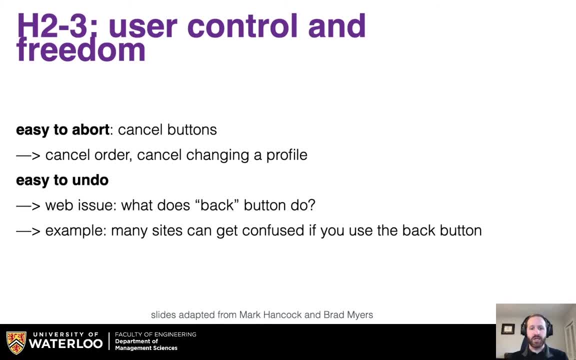 You have to keep in mind that users, even experts, will make errors. We need to design our system to either prevent those errors or allow easy recovery of them. There's no way to get out of editing a text field. then you're stuck in there you have. 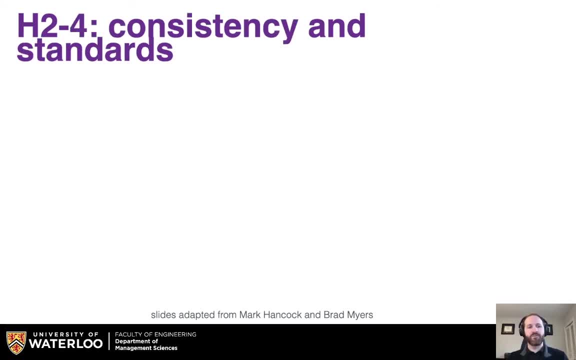 to put something in there. that's a problem. The fourth heuristic is consistency and standards. You want to have the same command always have the same effect. You want to have locations for information. Consistency of commands to give the user a mental model of the system. 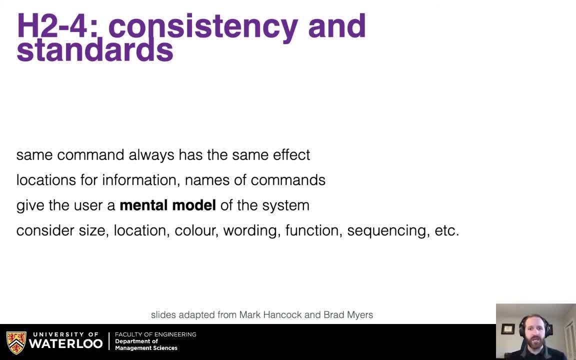 Consider things like size, location, color, wording, function, sequencing, et cetera in some of the ways that we've described for visual feedback. right And following standards can really help. If you follow existing standards, then it will be standardized. it will follow what. 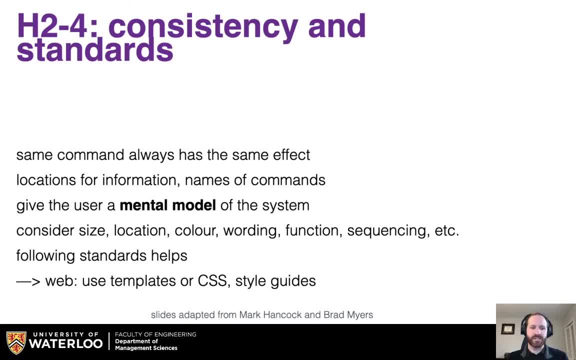 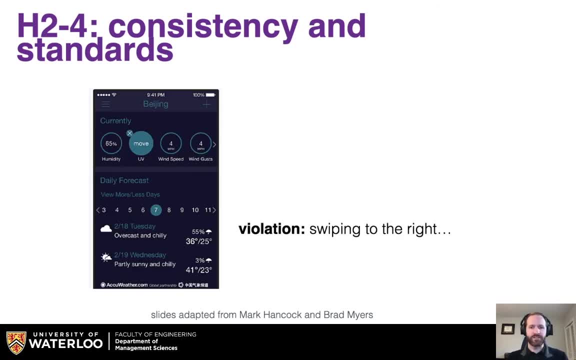 other systems are doing So. for the web, you might want to use templates or CSS style guidelines to make sure everything is relatively consistent. So, for example, this weather interface right here, It's a violation. If you swipe to the right, it changes the day. if you go slow and changes the city. if 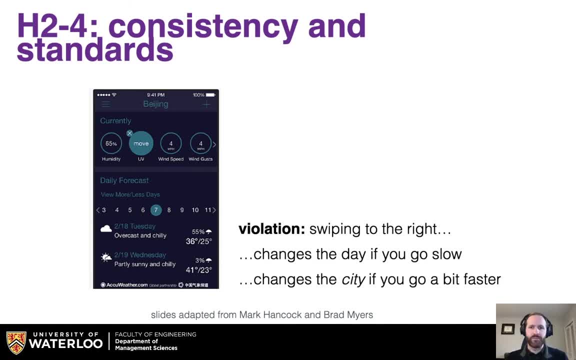 you go a bit faster. Sure, this offers a bit of control, but there's no way that would map to a mental model for me, right? I would imagine if you go slowly and change the day and you go quickly, maybe do a week. 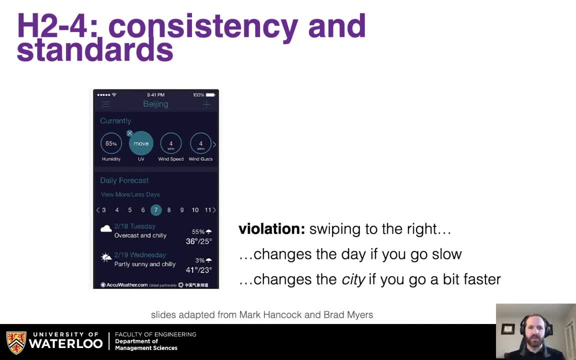 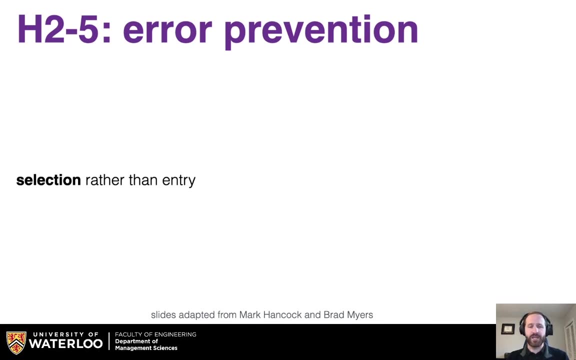 or maybe do several days, or start to roll and have momentum in a physical rendering somehow. But to actually change what it's scrolling between depending on the speed doesn't make sense. It's not consistent. The fifth heuristic is error prevention. Here you want to focus on selection rather than entry whenever it makes sense to do so.